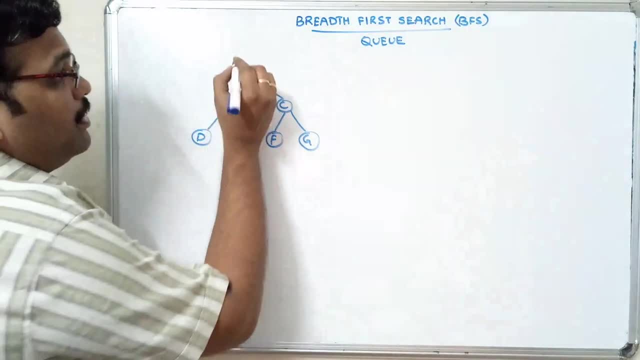 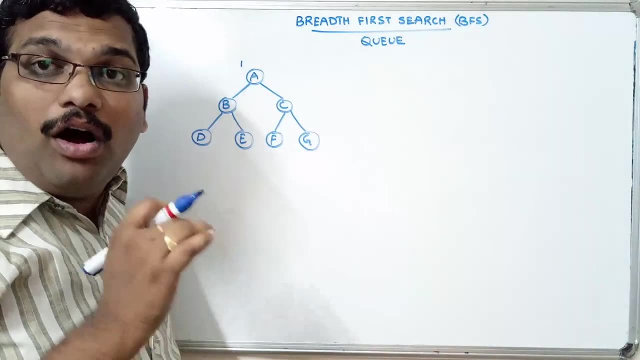 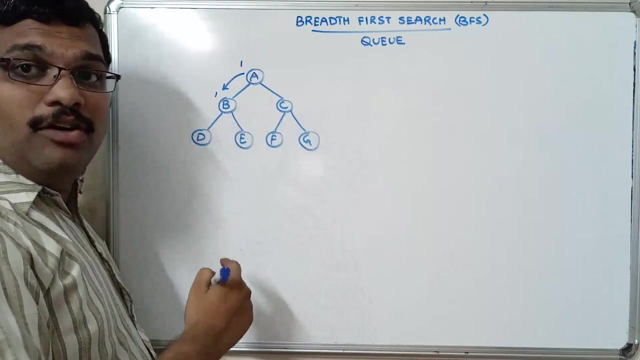 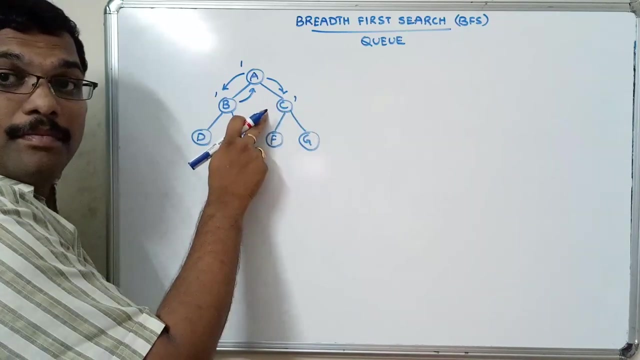 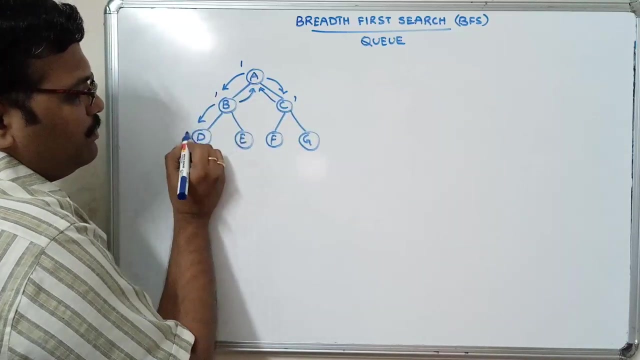 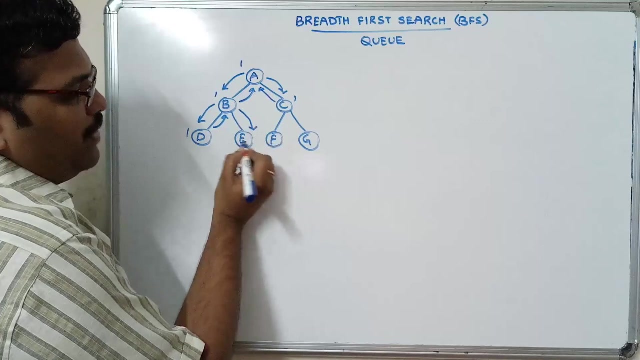 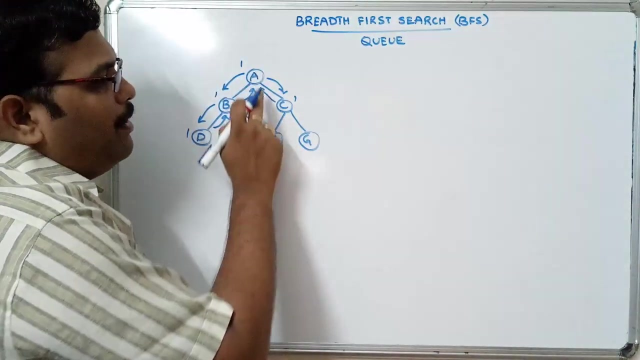 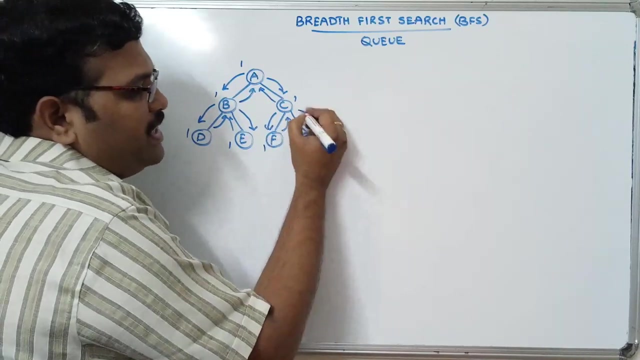 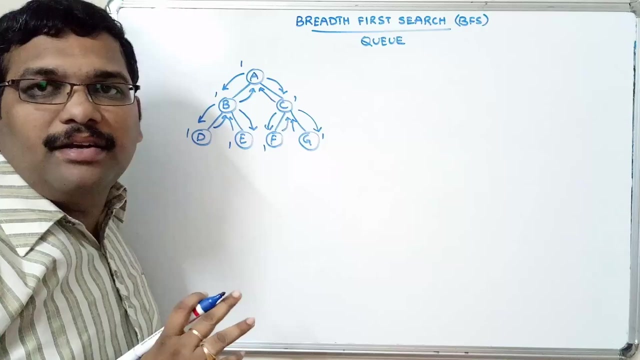 Right. So first travel from A, So mark it as one. So then visit the adjacent nodes, All the adjacent nodes. So first one, and there is one more adjacent node, One Right. Next level, visit the adjacent node of B and then visit the adjacent node of E, Backtrack Right, Because there are no adjacent nodes here. So backtrack to A, Again backtrack. Come to C, So visit F and backtrack to C, Visit G, Backtrack to C, Backtrack to A, So that all the adjacent nodes have been visited. 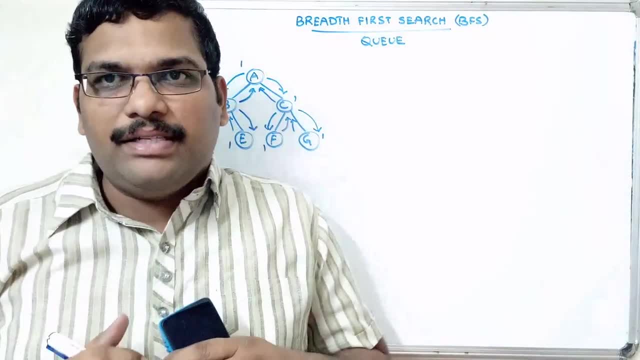 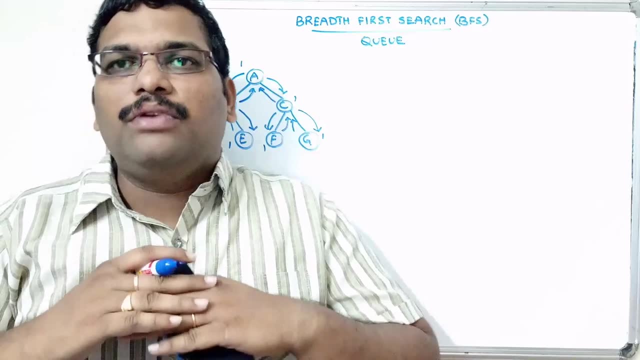 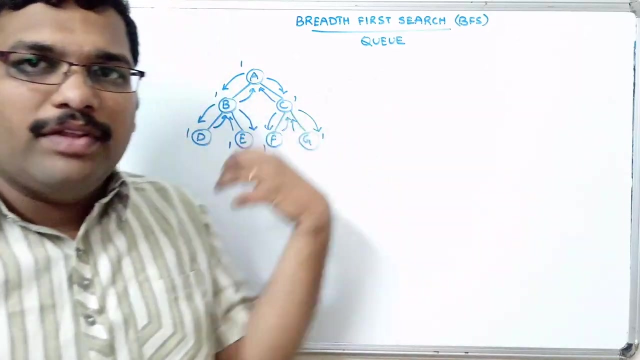 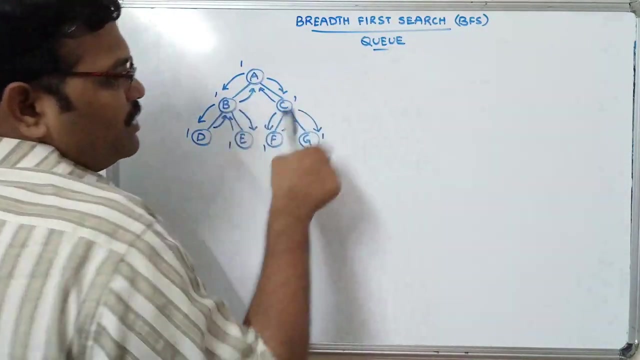 So here we have to visit the nodes in level wise. So first complete the level, Top level, Level 0. And then level 1, level 2, level 3.. So, top level, we have to complete all the visiting, all the nodes, Then go with the second level, Go with the third level. Now we will go with the implementation. So here, after visiting all these things, we will get the same order: A, B, C. 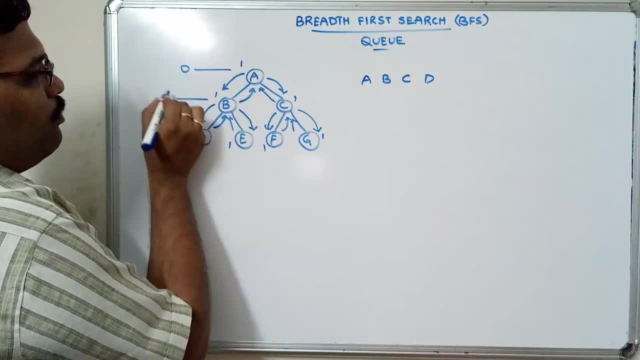 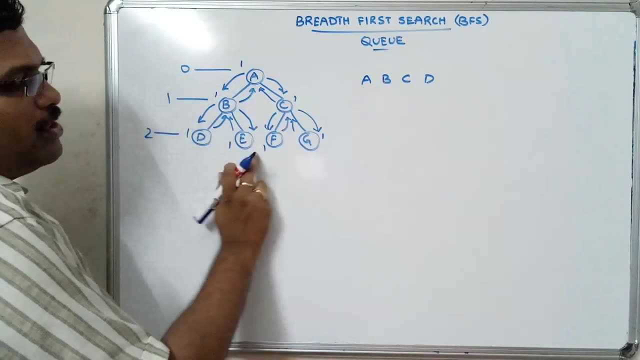 So A: Level 0.. Level 1.. Level 2.. So level 0. visit the node Level 1. visit all the nodes B, C. Level 2: visit all the nodes D, E, F and G. 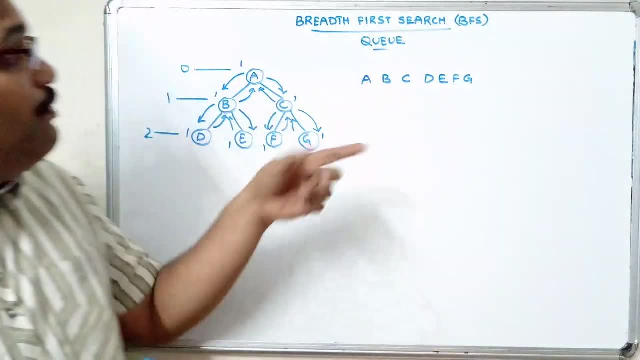 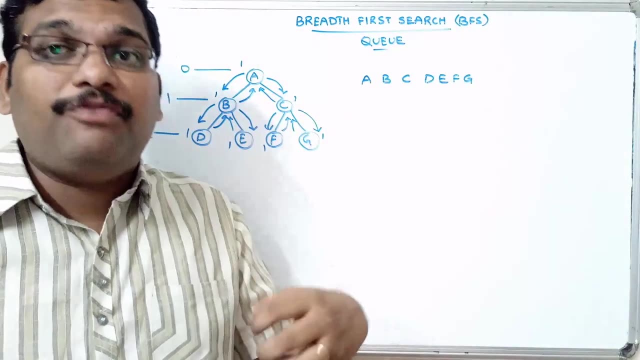 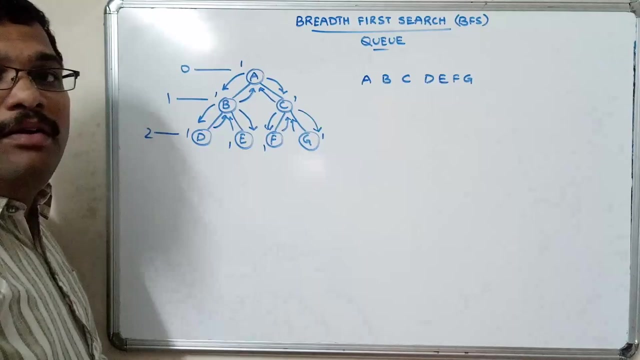 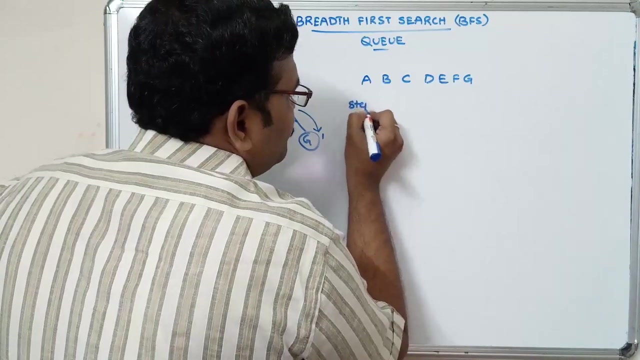 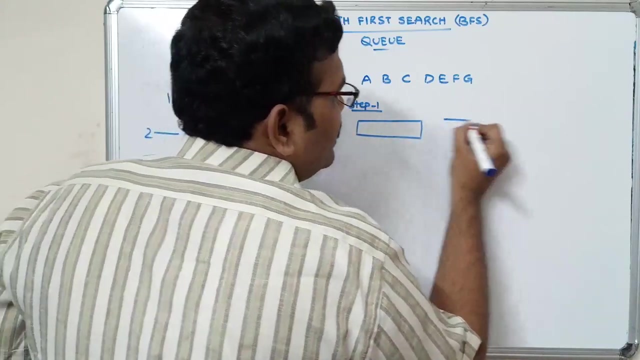 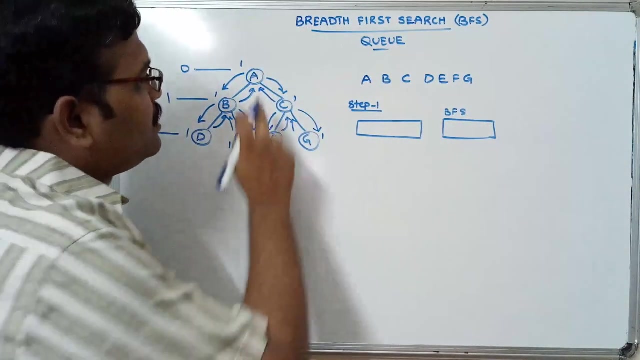 So we have to visit all the nodes level by level. So that's why we call it as a breadth first search. Okay, So in the previous session we have seen depth first search. We have to go in a depth. Now we will see how we will get this one with the implementation of Q. So step 1.. So this is a Q And this is a BFS, Q and BFS. So first let us assume this one is a start node. 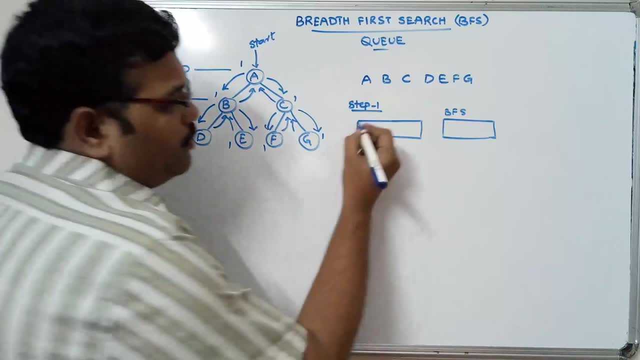 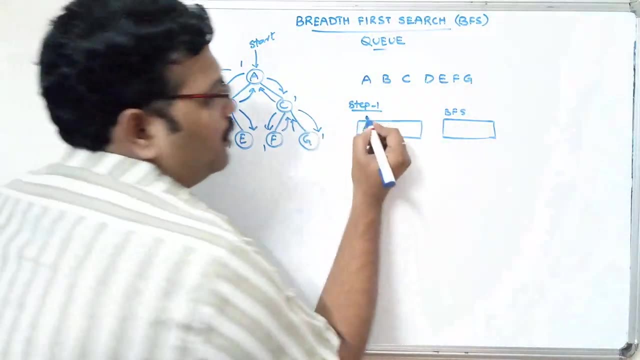 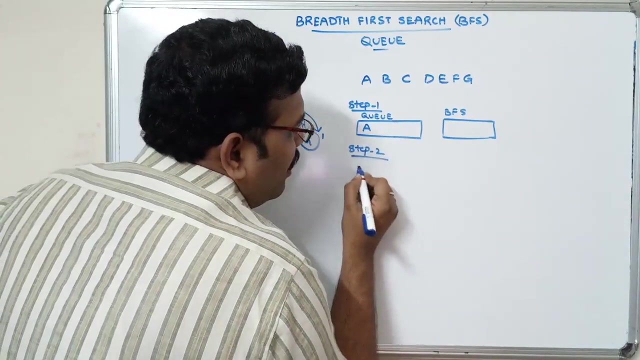 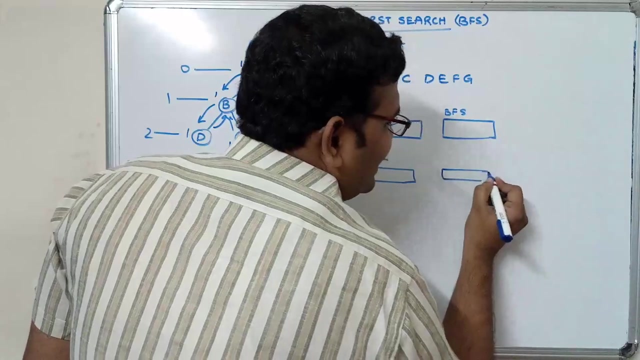 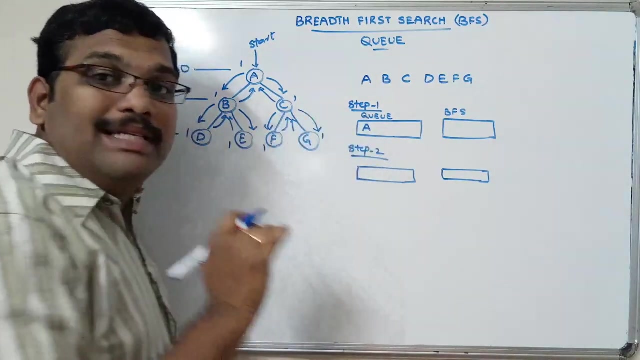 Okay, Same thing. Start node is so a right. insert a into the cube, so this is a cube. okay, step 2: remove the element from the cube and place in DFS, BFS. so as it is a cube where we have to remove the element, so both the insertion and deletion will be applied on same end. 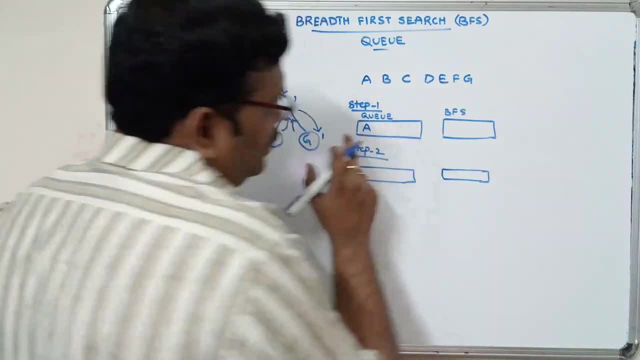 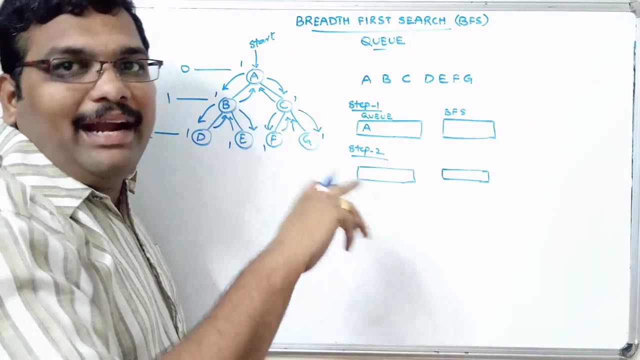 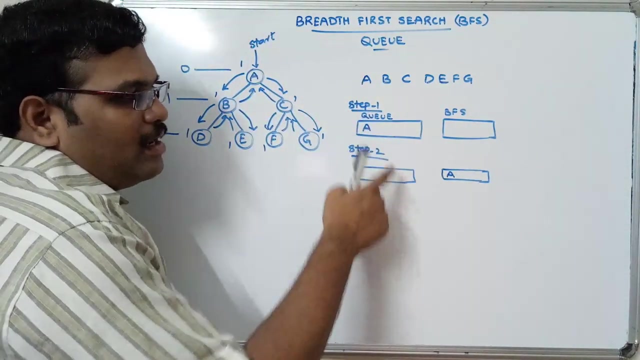 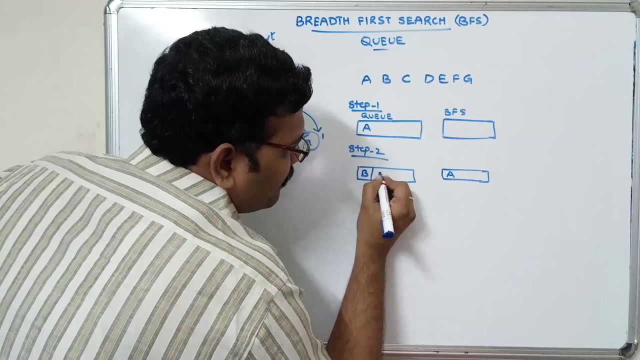 okay, so sorry. so deletion will be from front end, insertion will be from back end, right, okay? so yeah, yeah, is removed and placed in BFS. now insert all the adjacent nodes of a in Q. what are the adjacent nodes in PA, B, C, B and C? so this: 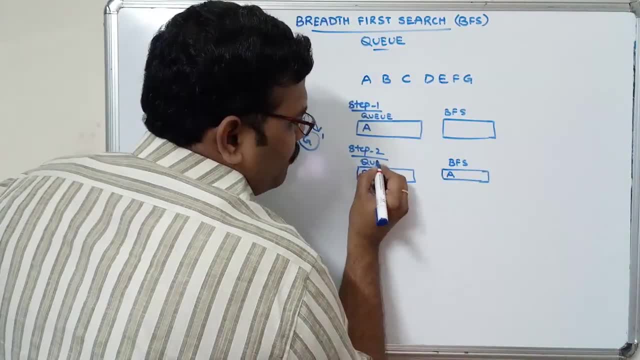 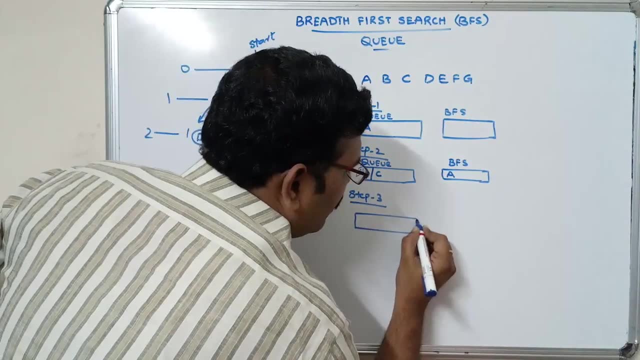 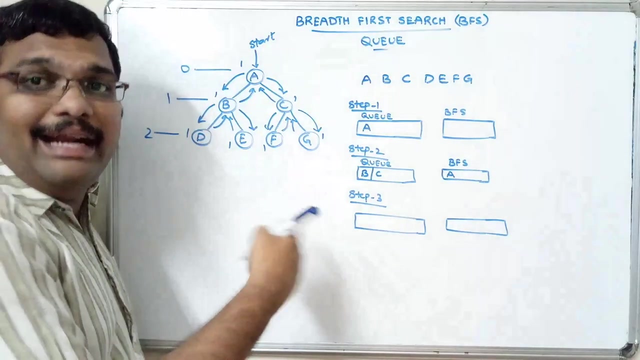 is a BFS and this is a cube. so in the step 3 and remove the element from the cube. so here we have to remove the element from the front end. we have to insert the element at the rear end. okay, so we have to remove the element, so the C will be in. 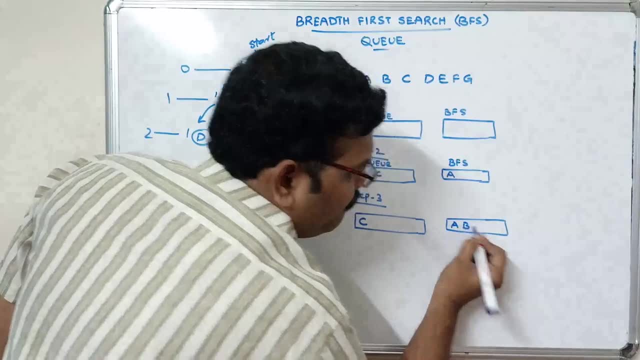 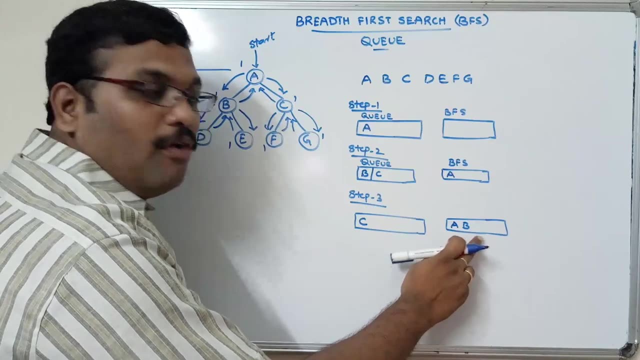 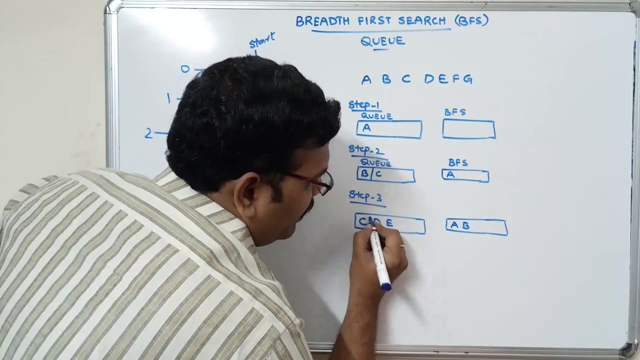 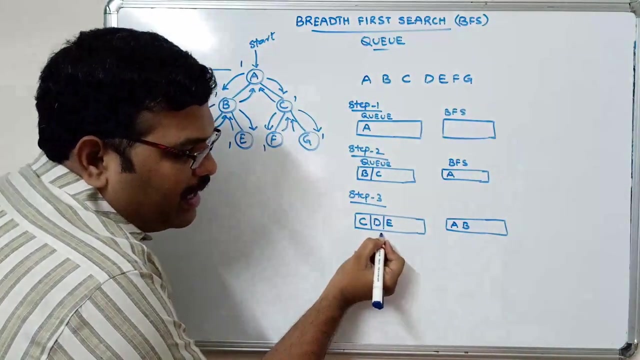 the top and place here a big. now what we have to do? we have to insert all the adjacent nodes of B into the cube. what are the adjacent nodes of B? D and E? so D, E. so how the insertion will takes place at the rear end. so this is a friend. at the rear. I have inserted D and next at the rear. 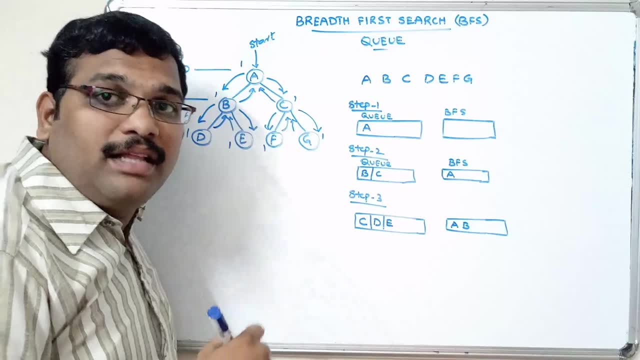 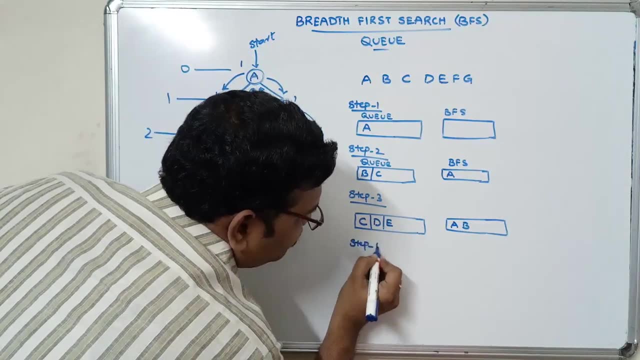 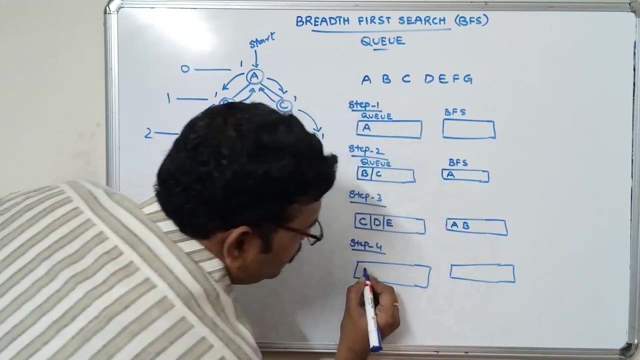 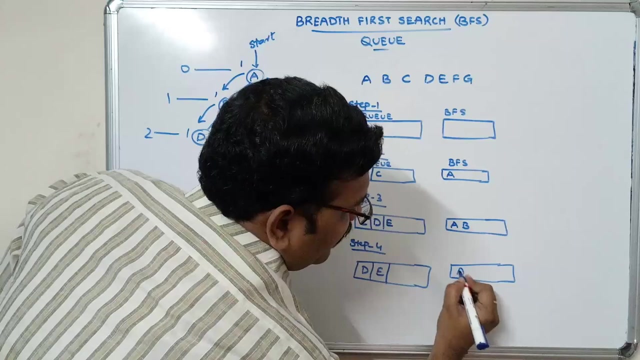 have inserted the E, so at the rear end I am inserting the nodes, adjacent nodes of B, because we are removing B here. next, in the step 4, remove the element from the cube. remove the element from the cube, so C is removed, because the element is deleted from the front end. so D, E, A, B, C. now what is the? 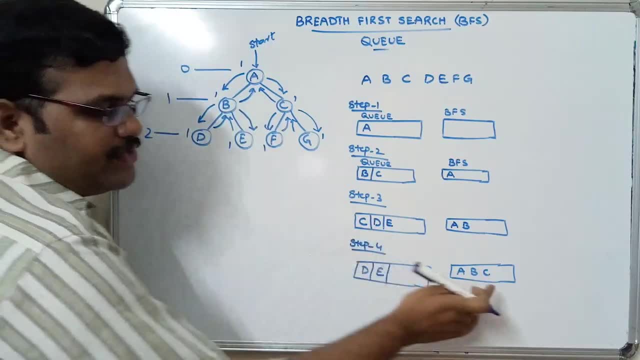 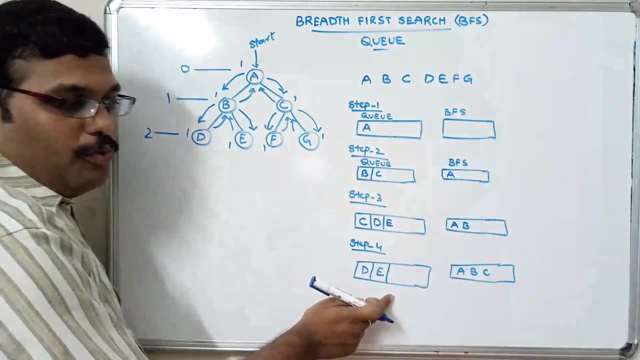 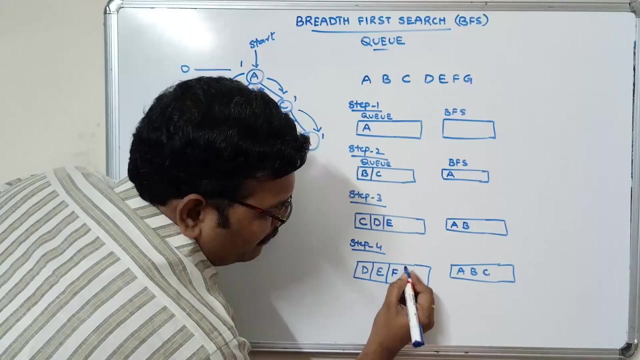 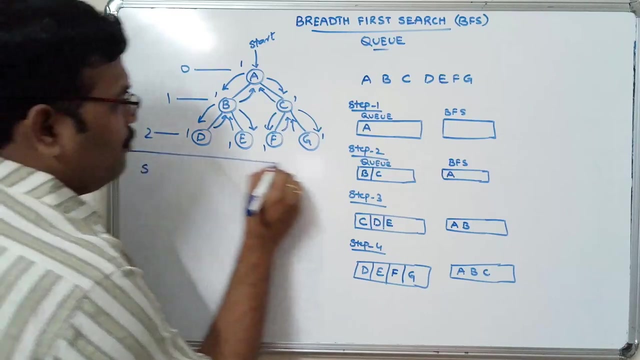 element. we have removed C. now place the adjacent nodes of C into the cube. place or insert the adjacent nodes of C into the cube, because we are removing the C from the cube. so what are the adjacent nodes of C, F and G? so insert them into the cube. F and G. so apply the same procedure. step 5: 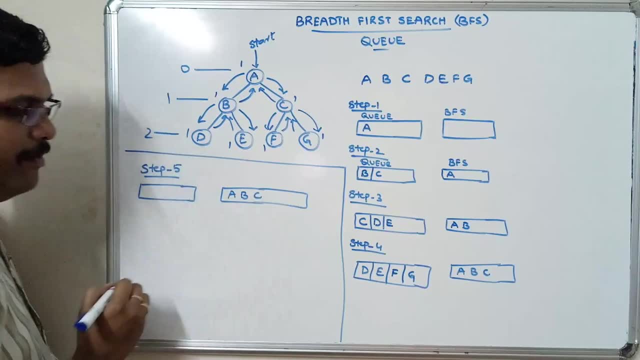 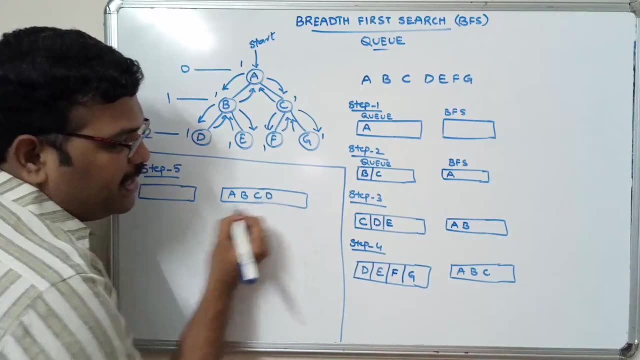 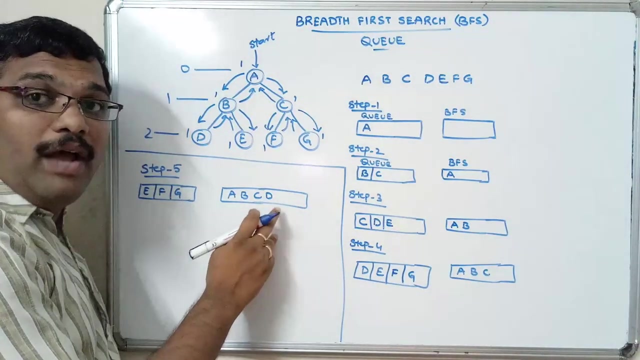 right. so already A, B, C are there. now remove the element, so delete. the deletion will be done from the front end. so D is deleted and placed here. now there are only three elements: E, F and G, and we have removed D, so we have to add the adjacent nodes of D into the cube. so here D is an if node, so here D doesn't. 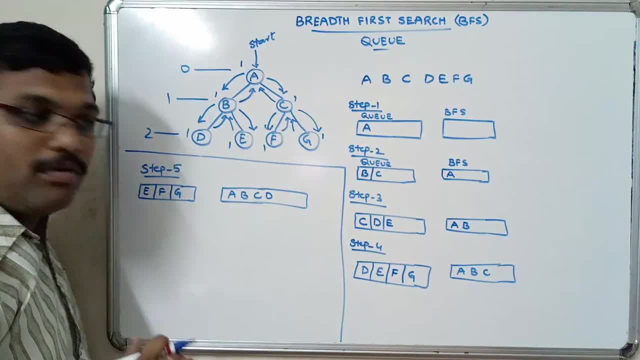 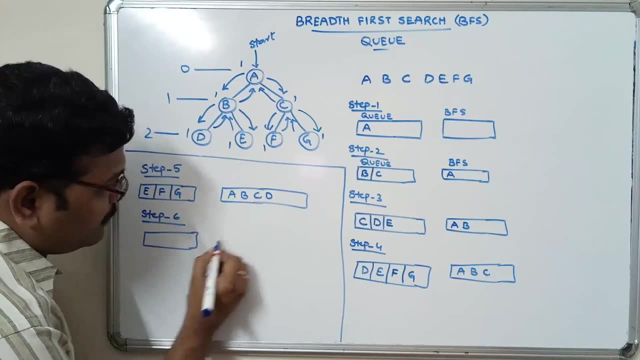 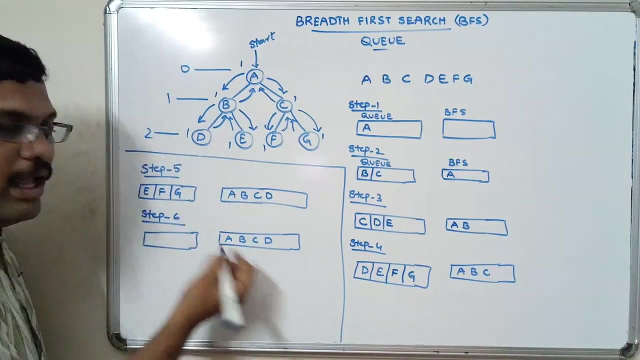 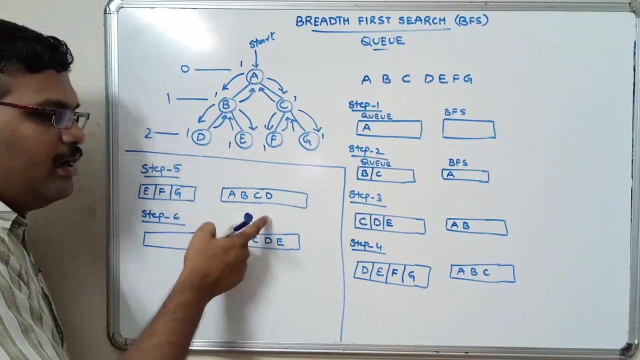 have any adjacent nodes, so just ignore. next, follow the same procedure, step 6. so A, B, C, D and remove the element. so element is removed from the front end, so E will be removed and we have to insert all the adjacent nodes of E into the cube. so what are the adjacent nodes of E? there are no adjacent nodes. ignore. 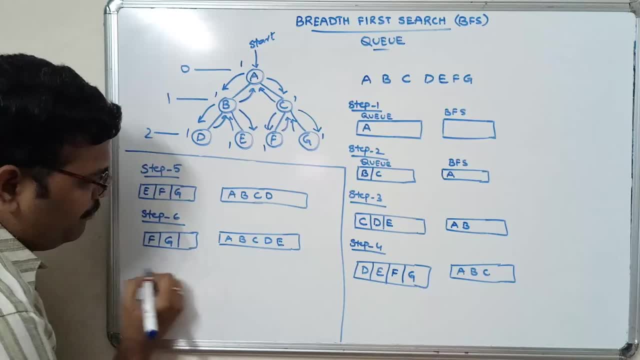 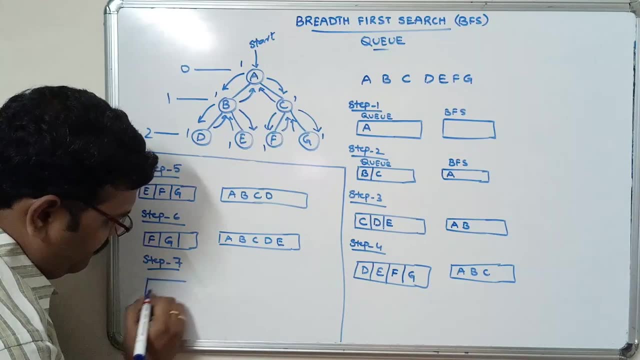 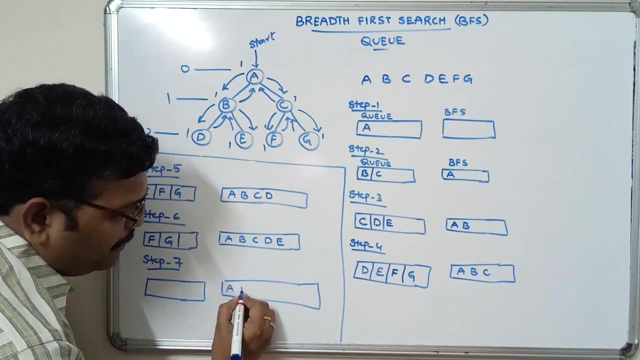 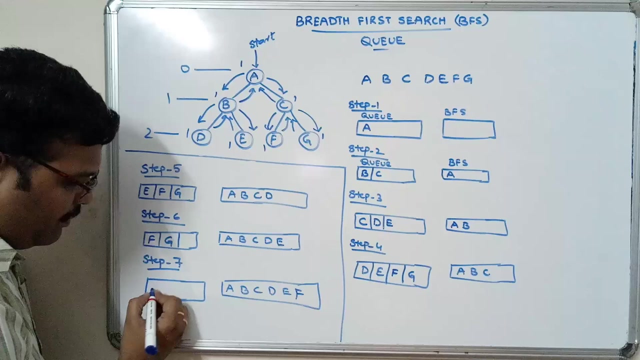 so there are only two elements in the cube. step 7: remove the element from the cube. step 7: remove the element from the cube and place it in the BFS. so what is the element F is removed here and placed in BFS, and we have to insert all the adjacent nodes of F. 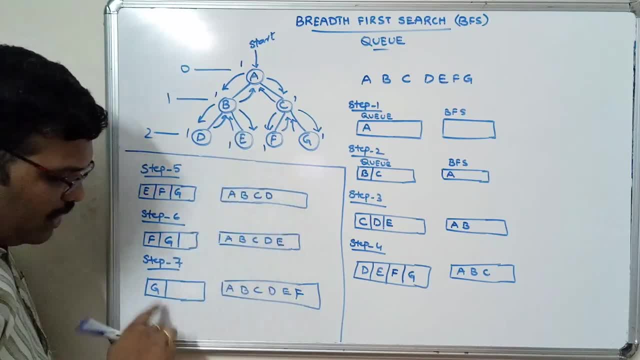 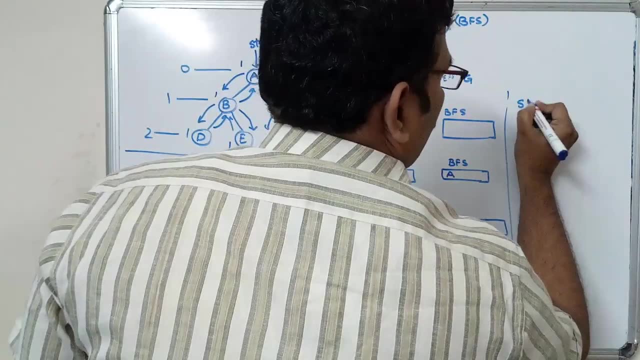 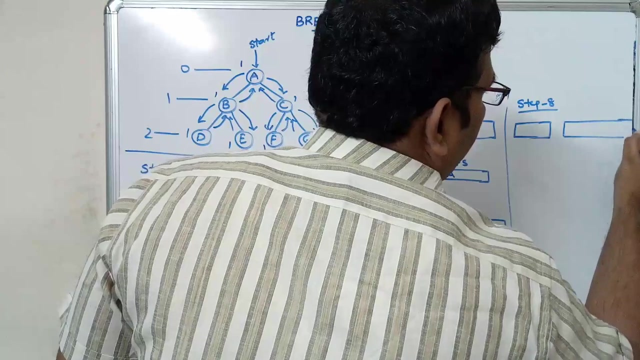 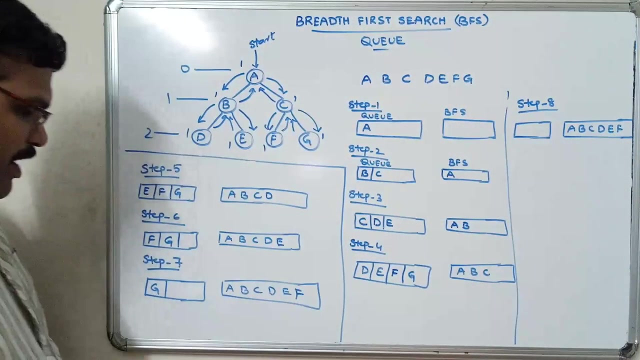 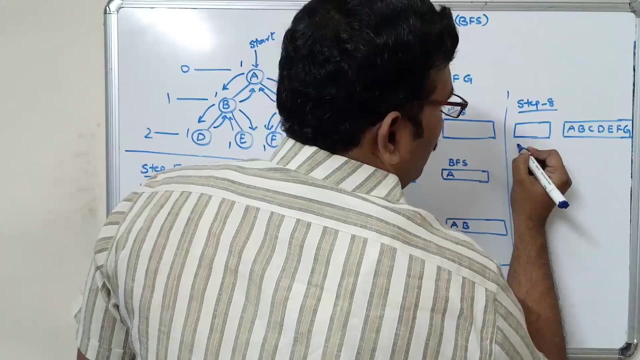 into the cube. so there are no adjacent nodes for F, so remove, just remove. next step 8, step 8. so A, B, C, D, E, F. so G is removed, so G is placed here and we have to insert all the adjacent nodes of G into the cube. so there are no adjacent nodes for G, so here Q is. 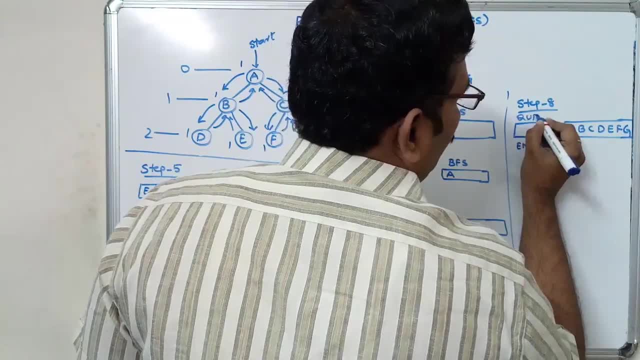 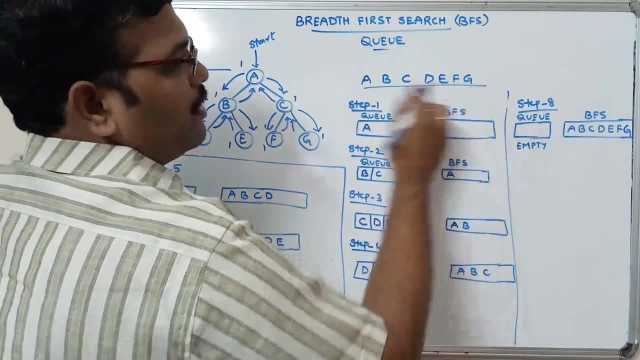 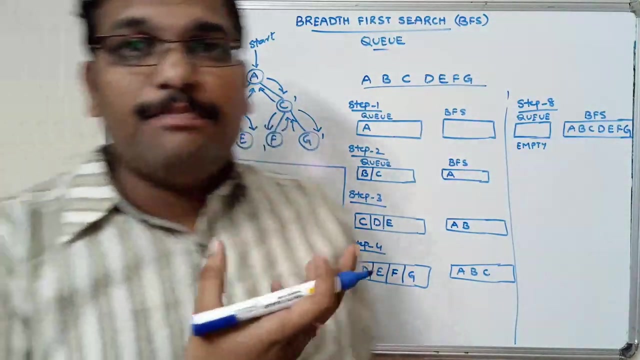 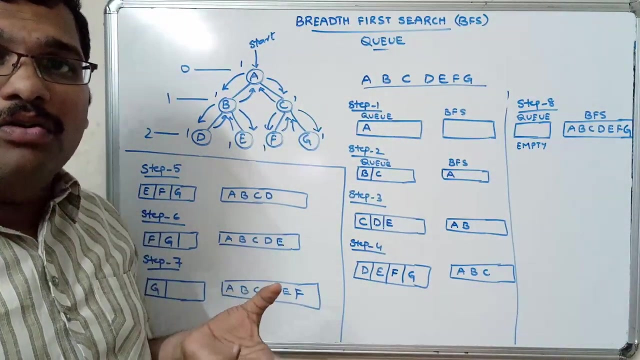 empty. so this is the cube and this is the BFS. so the same thing we got here: A, B, C, D E, F G. A, B, C, D, E, F G. so this is how we can implement the BFS breadth: first search using Q. so hope you understood. so here we are visiting all the nodes level by level. so we have to. 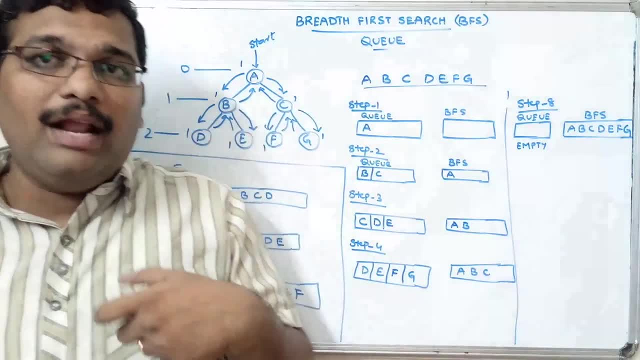 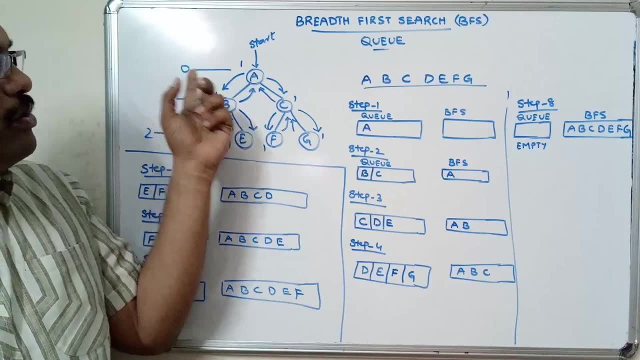 visit all the nodes in level 0, then only we have to go with the level 1, then only we have go to the level 2, right? so here, A in level 0. so we have visited A in level 0 in the level 2, sorry, level 1. 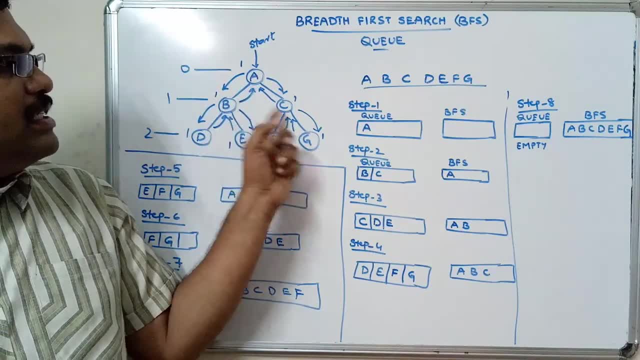 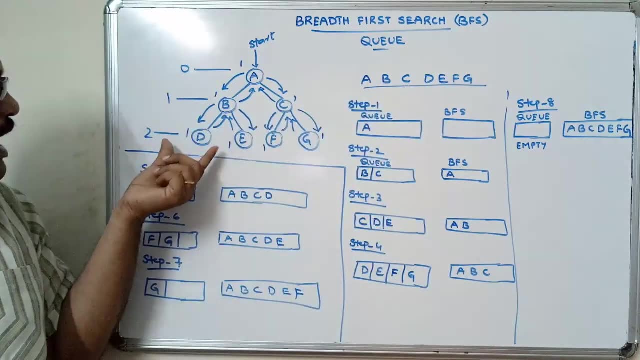 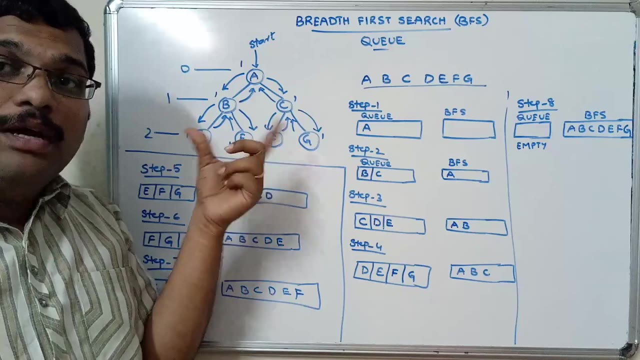 there are 2 nodes which are adjacent og A, so A, B, C. so we have visited B and C and then we will go with the level 2, because only 2 nodes are there in level 1. in the level 2 there are 4 nodes and we have to visit all this 4 nodes before entering into the next. 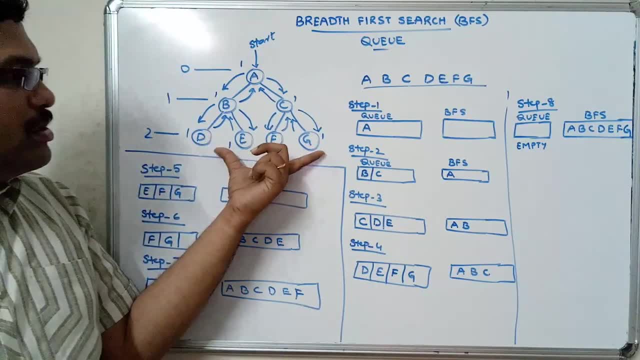 level. so visit all these nodes because all this nodes are adjacent to the the same level. we would have to go like this thing again. so before invoking all this nodes now, what we have to do is justолж go with the level 2 science and pump it like this and in the next level. 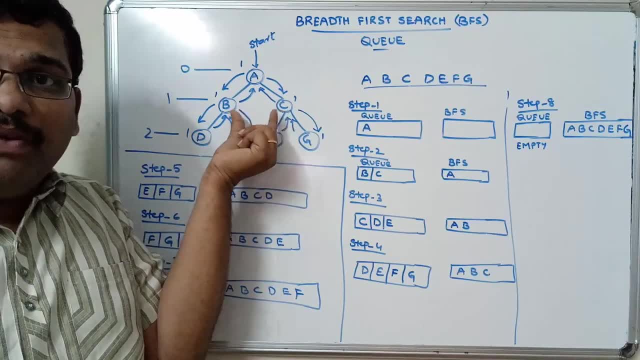 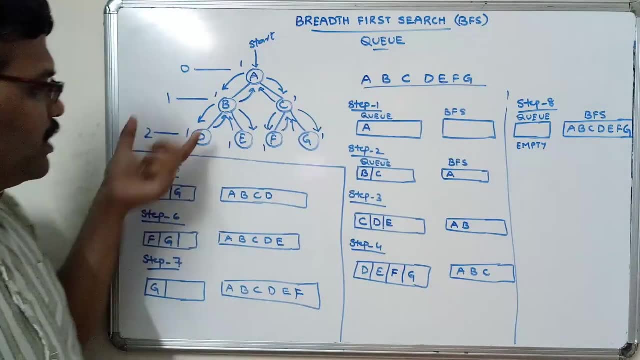 we will just go to see the next level and during this path we will going to visit the next left to B and C, all the nodes of level 1, so D E F G. so we are visiting D E F G and go with the next. 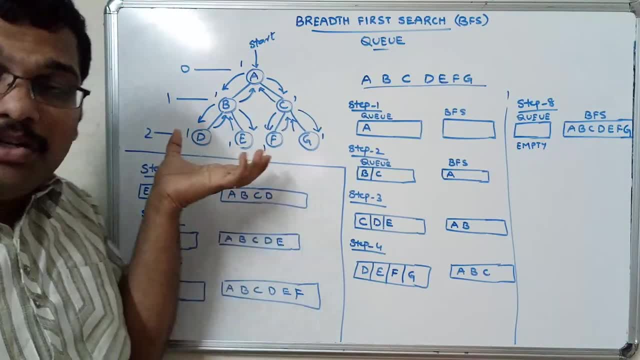 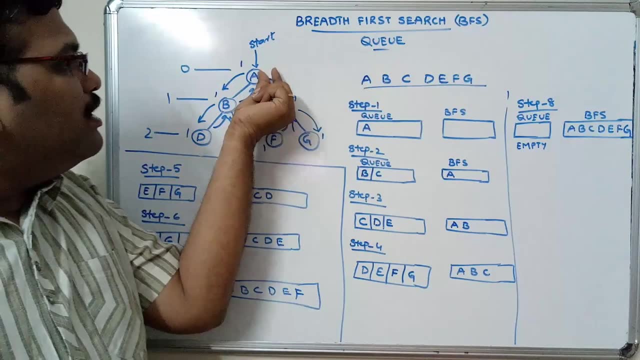 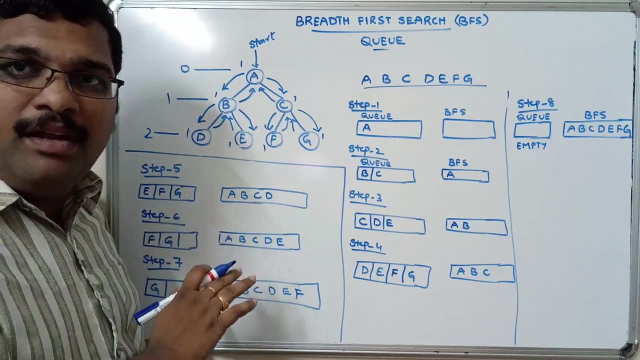 level. so there are no other levels, right, because level 2 is a last level. so this will be the answer and this will be implemented by using the queue. just insert the node into the queue and then first insert the node into the queue if the queue is empty. if not, remove the element or remove that. 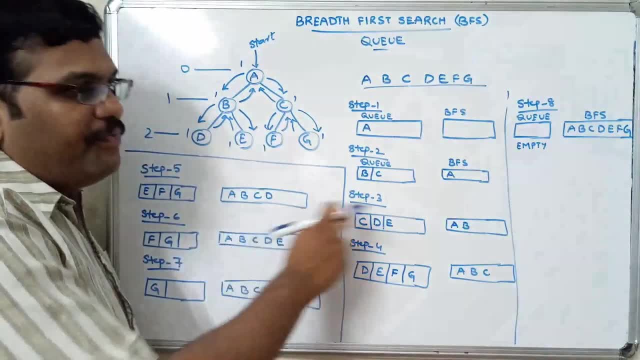 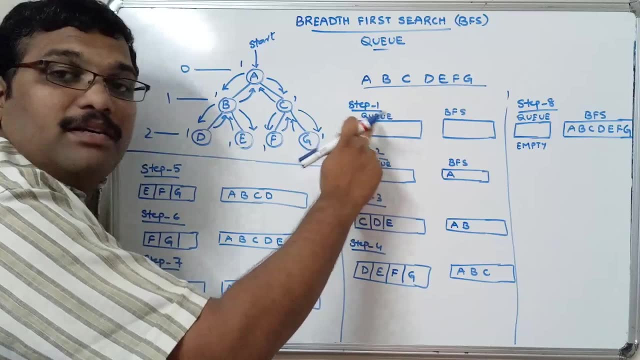 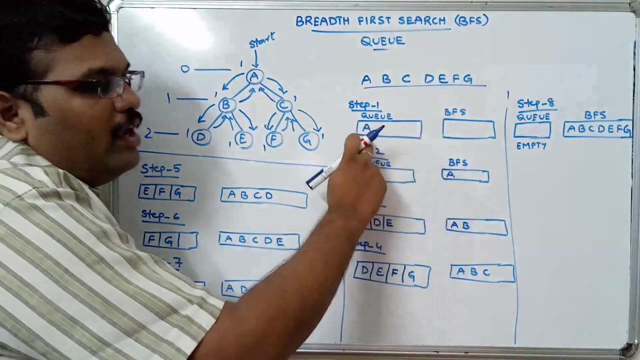 node from the queue and enter into the BFS, place it in the BFS and insert all the adjacent nodes of that particular node into the queue and follow the same procedure. so first we have inserted A and then we have removed the A and placed it in the BFS and we are. we have to insert the elements. 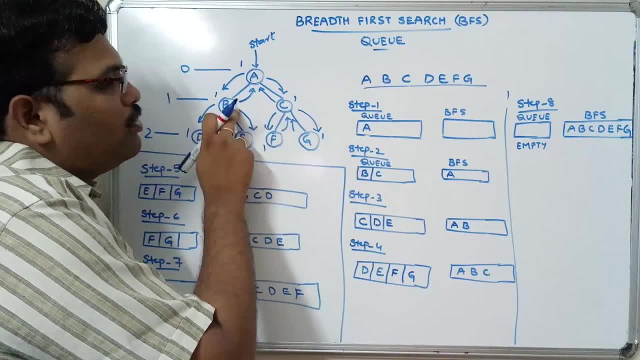 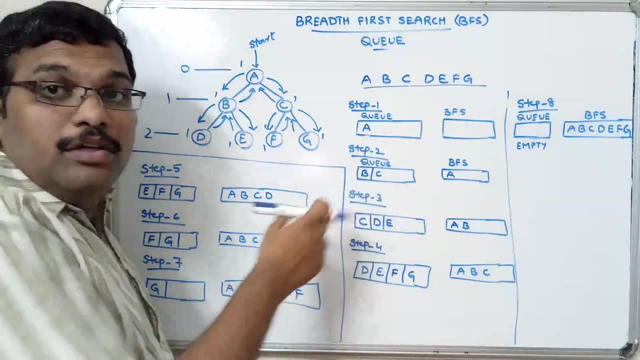 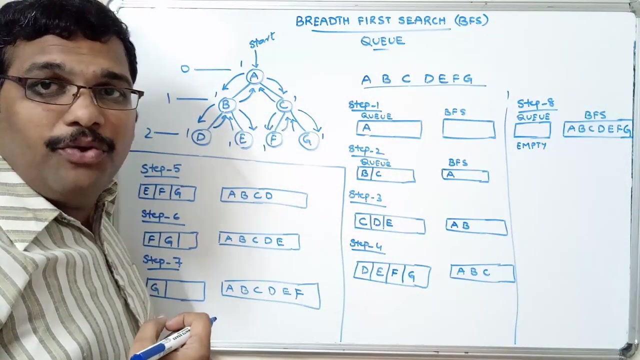 of adjacent nodes A into the queue. there are two adjacent nodes, B and C. so B and C, right in the next step we have to remove the element from the queue. so where we have to remove the first element from the front end. so from the front end we will remove the node from the queue and will insert.